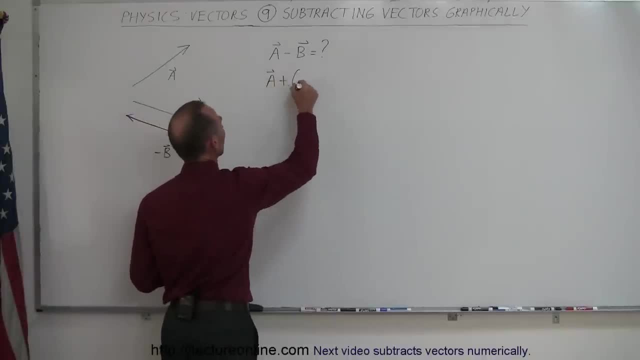 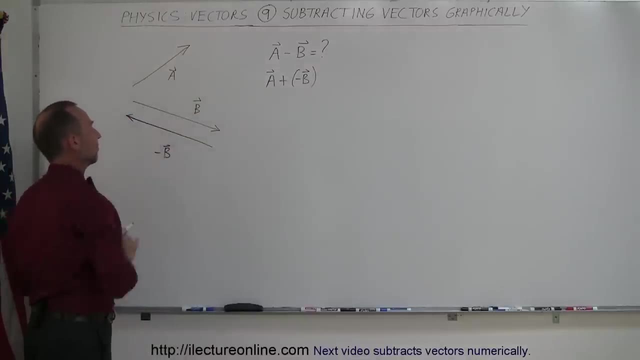 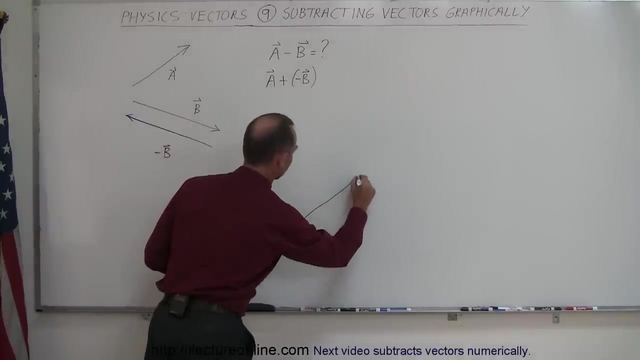 to. I can change this to A plus negative B, And then all I have to do is simply add this A vector to this negative B vector, and so what I can do then is redraw vector A over here. So there's my A vector. I'm going to add my negative. 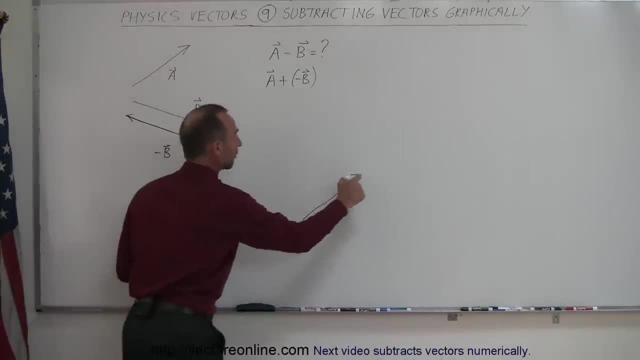 B vector. so I'm going to put the tail of the B vector on the tip of vector a. take this, put it over here, and this is my negative b vector. and so now i know that when i add those two together i get the resultant. so this here: 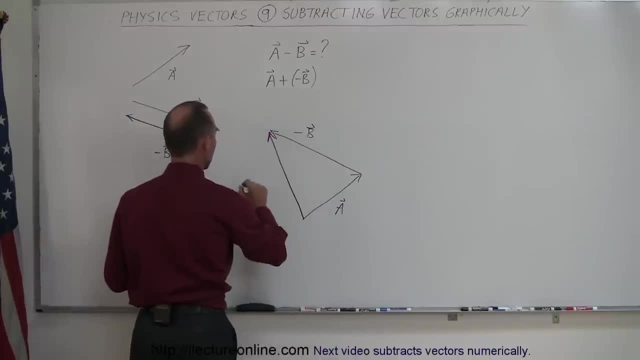 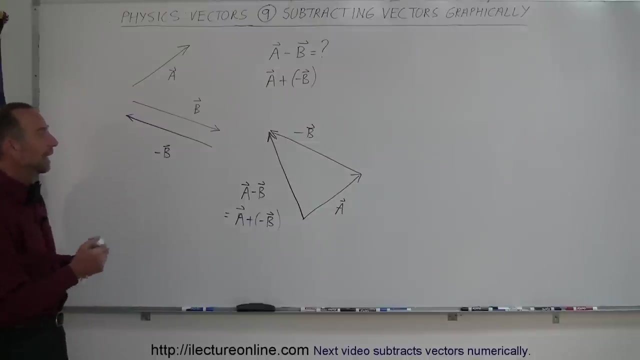 is my vector a minus b or a plus or a plus the negative b vector? all right, that's how we subtract vectors. we simply find the negative of the second vector and then add that to the first vector to get the difference of two vectors. and that's how you subtract vectors graphically. 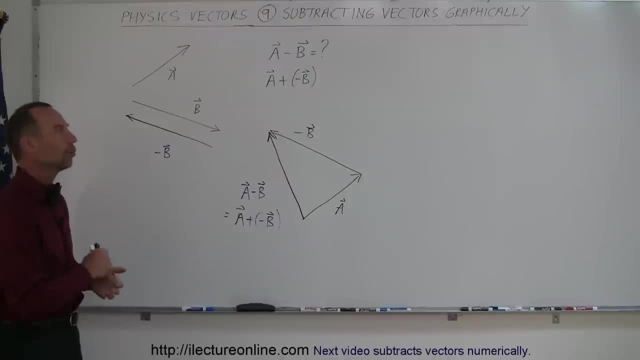 in our next example, we're going to show you how to do that same kind of thing numerically as well. 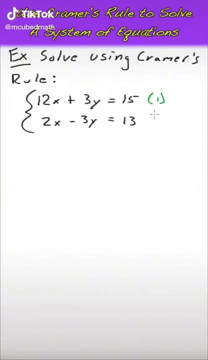 Let's solve the following system of equations using Kramer's rule. Kramer's rule states that the solutions are a ratio of determinants of matrices. The denominator matrix D has the coefficients of x in the first column and of y in the second column, so 12,, 2, and. 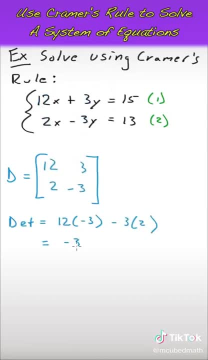 3, negative 3.. Computing the determinant gives negative 42.. Then dx is similar to d, but swaps the constant terms in for the x values, so 15,, 13, and 3, negative 3.. Computing the determinant gives negative 84.. Dy is also similar to d, but swaps the y values, so 12,. 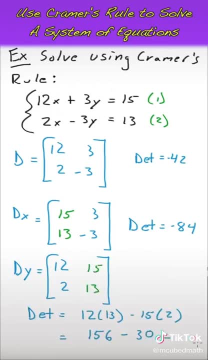 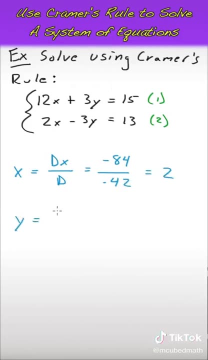 2, and 15, 13.. Computing the determinant gives 126.. Finally, x is the ratio dx over d, which reduces to 2,, and y is the ratio dy over d, which reduces to negative 3.. Thus our 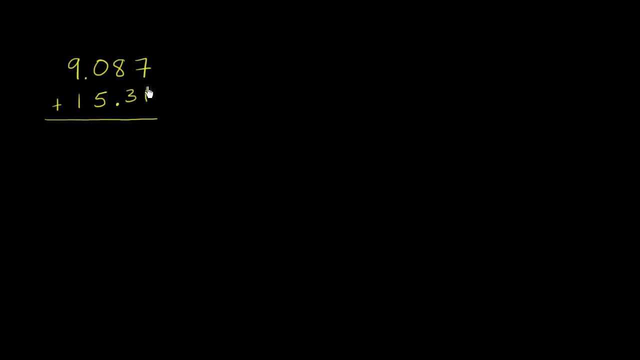 Let's see if we can add 9.087 to 15.31. And I encourage you to pause the video